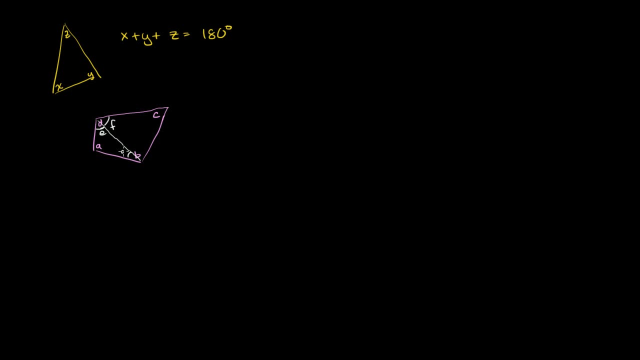 Let's call this angle over here f. Let's call this angle over here g. Let's call this angle over here h. So we know what we're trying to find is a plus b plus c plus d, But we know that b is the same thing as g plus h. 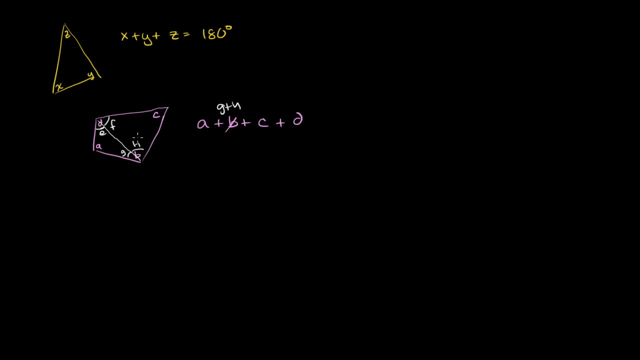 b is the same thing as g plus h, And we know that d is the same thing as g plus h. d is the same thing as e plus F, And the reason why this is interesting is we then see that the sum of the angles in each of these triangles 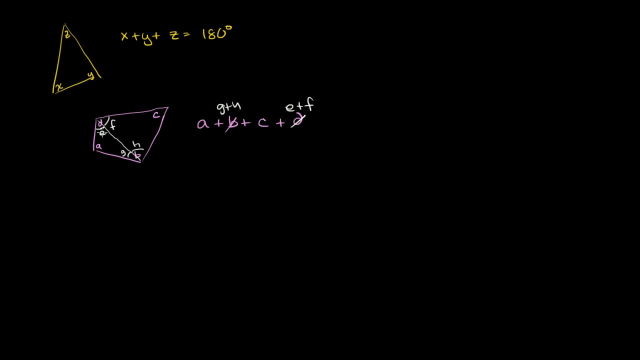 are going to be equal to the sum over here. So we know that a plus e plus g is equal to 180 by the same exact idea up here. So we know that a plus g plus e is equal to 180 degrees. a plus g plus e is equal to 180 degrees. 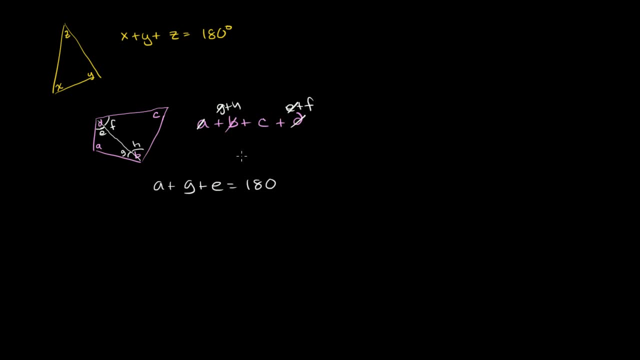 Now here, begin with this: 1 minus A plus g plus E is equal to 180 degrees. 180 degrees. So you take those out, you're left with 180.. And then we also know that F plus H plus C is equal to 180 degrees. 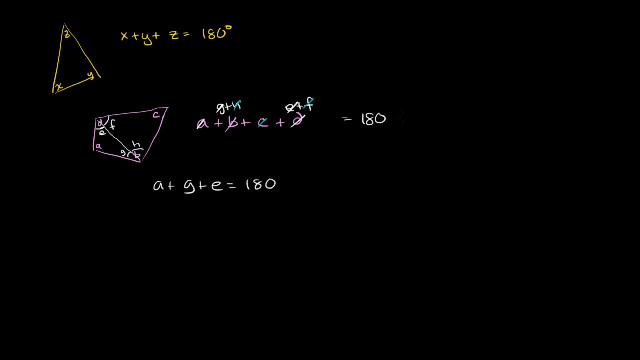 F plus H plus C is equal to 180 degrees. So it's equal to 180 plus 180, which is equal to 360 degrees. So the sum of all of these interior angles, the measure of all of these interior angles, was equal to the sum of all of the angles. 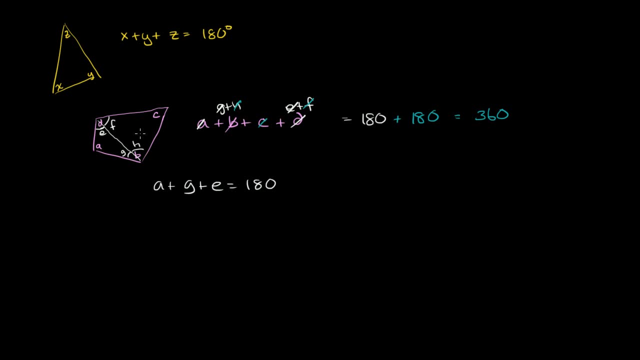 of each of these triangles, these non-overlapping triangles that I divided it into. So the real crux: if I look at an arbitrary polygon, let's look at a hexagon here And it won't even be a regular hexagon. 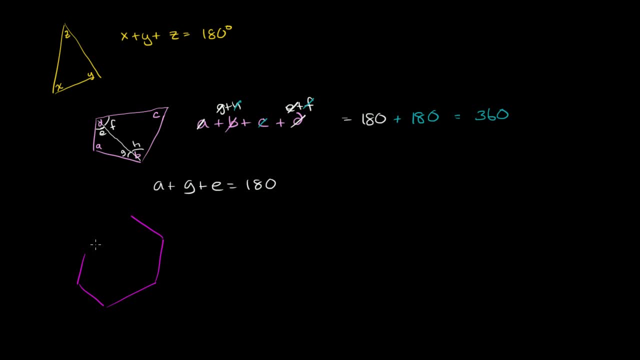 1,, 2,, 3,, 4,, 5, and 6 sides. So this is a very irregular hexagon, But once again we can do the same logic. What is the sum of It's interior angles? 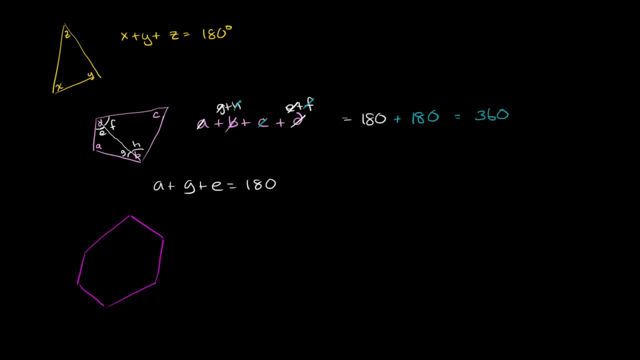 We'll just divide this hexagon into triangles, non-overlapping triangles. So this could be one of the triangles, That could be another of the triangles, That would be the other triangle, And then we have this fourth triangle right over here. So we have 1,, 2,, 3,, 4 triangles. 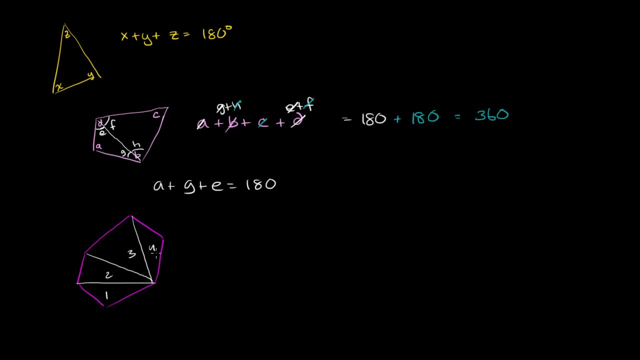 And then the sum of the angles in each of those four triangles is 180 degrees. So the sum of all of these angles, the sum of this angle, that angle, that angle is going to be 180.. Then you have this angle: 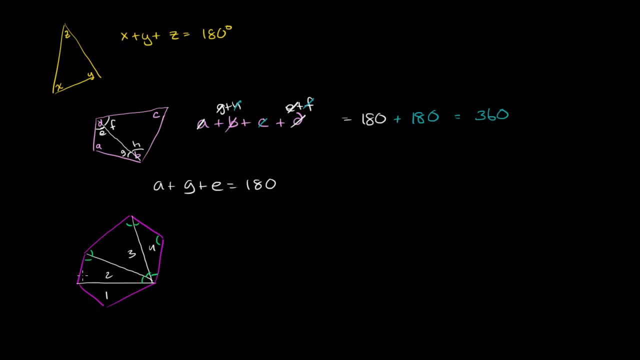 This angle, That angle is going to be 180. Then you have that angle, That angle, That angle is going to be 180. And then that angle, that angle and that angle is going to be 180. And I think what you just saw me do. 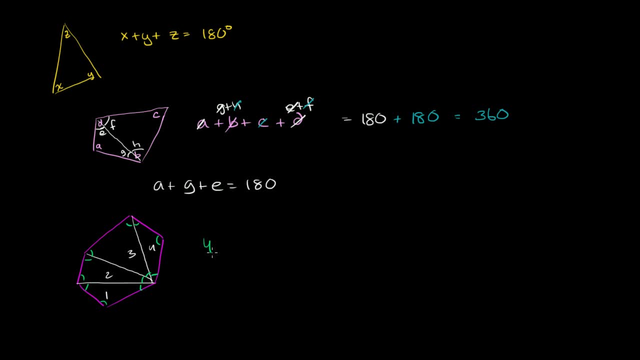 is I'm essentially going to have 4 times 180 degrees is the sum of all of these green angles that I drew here. But the sum of those green angles is also going to be the sum of the interior angles of this hexagon, Because the sum of these four is this one right over here. 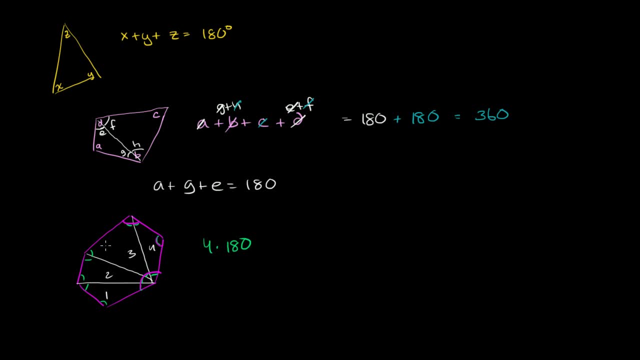 That one is that one, Then those two are those That interior angle. That interior angle is the sum of those two angles. That interior angle is the sum of those two angles. So we get 4 times 180, which is 640 degrees. 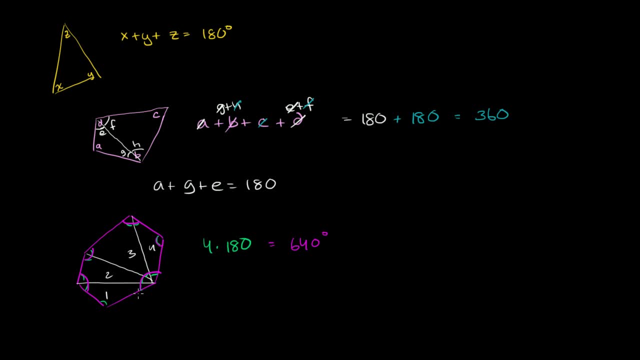 So the general idea is you just want to split your polygon into non-overlapping triangles, And however many non-overlapping triangles you can split it into you, just multiply that times 180 degrees And that will be the sum of the interior angles. 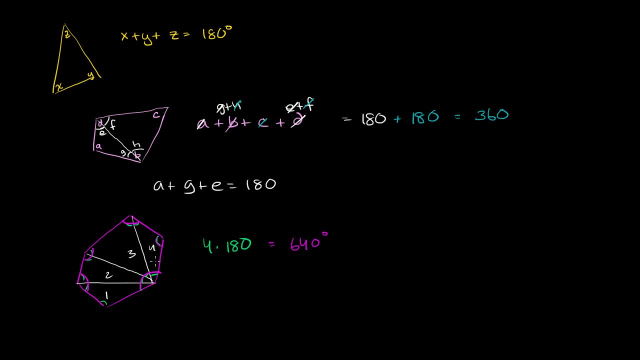 So the next question you might say is: well, OK, That's pretty quick, I can divide things into triangles pretty fast, But is there a general way of thinking about how many triangles I can divide something into? We know that one triangle can only. 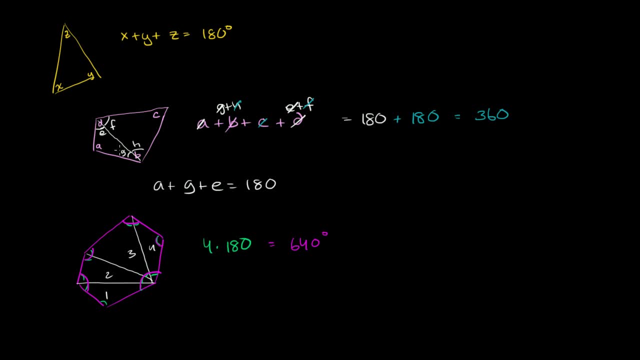 be divided into one triangle. We know that a quadrilateral can be divided into two triangles. We know that a hexagon can be divided into four triangles. Is there a general- and you might already be sensing a general pattern here: if we have an n-sided polygon, how many triangles? 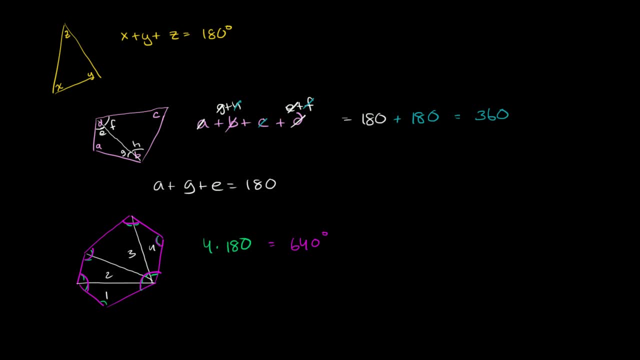 can I divide that into? So let's think about that a little bit. And just for the sake of argument, let's just assume that n has more than 180 degrees, More than 4, that n is greater than or equal to 4,. 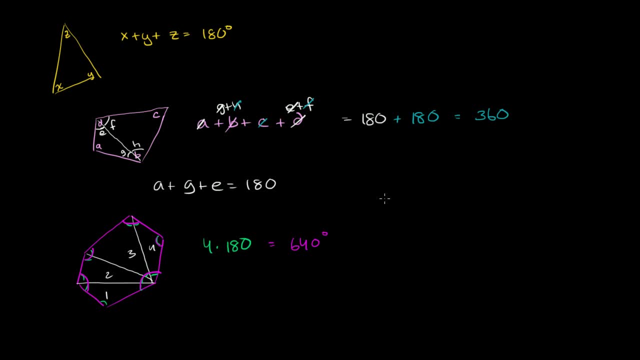 or actually greater than 4.. So what happens is: so let me draw it like this. So I'm going to draw my arbitrary polygon like this, So I'm going to draw two of the sides right over here, And then I'm going to draw two of the sides over here. 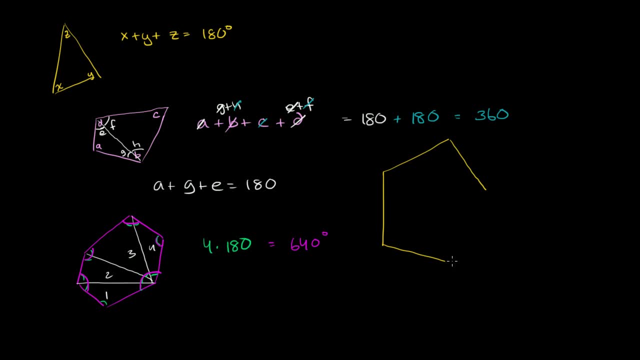 And then we don't know what's going to happen here just yet. So there's all sorts of, let's say, assuming that I covered this up with black construction paper, there might be a ton of sides right over here. Remember, these can be irregular. 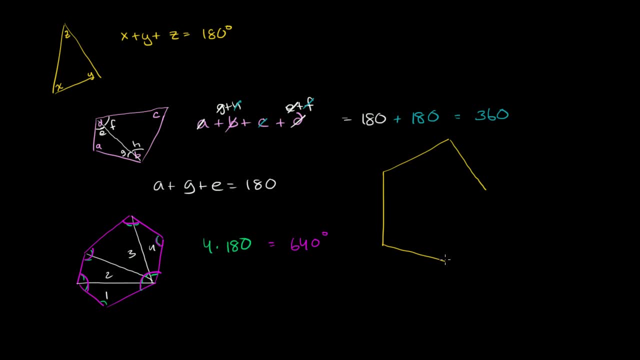 It might look like that. In fact, I could put an infinite number of sides here depending on. I can make it do all sorts of. I can make it do all sorts of crazy things to put a bunch of sides right over here. 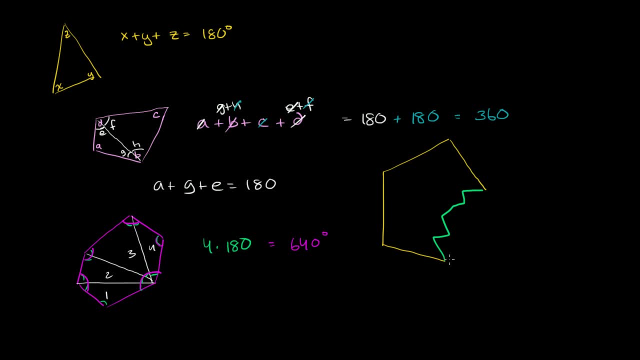 And you can imagine it creates a very irregular polygon. But let's just worry about what we can see. Well, these four sides right over here. I can make two triangles out of them, One like that and then one like that. 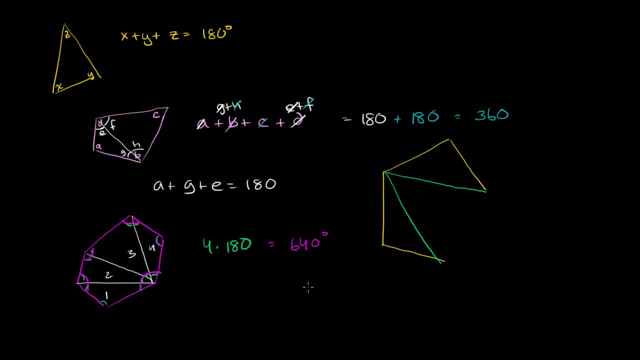 So we know, regardless of however many sides this has. so if this has n sides, if we have n sides right over here, we can use four of the sides to come up with two triangles. We can use four of the sides to come up with two triangles. 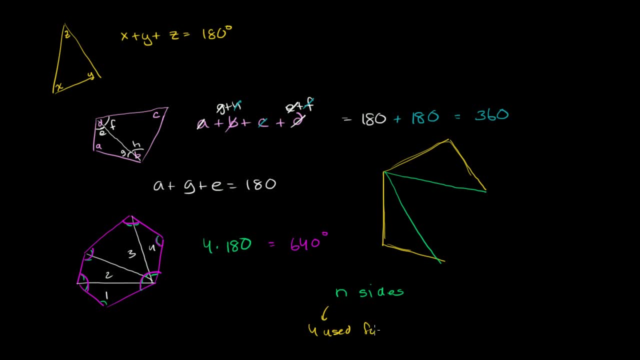 So four used for two of our triangles. And then how many triangles can we make with the remaining sides? So let's just imagine different things. So let's just imagine every remaining side other than these first four. I can make another triangle with. 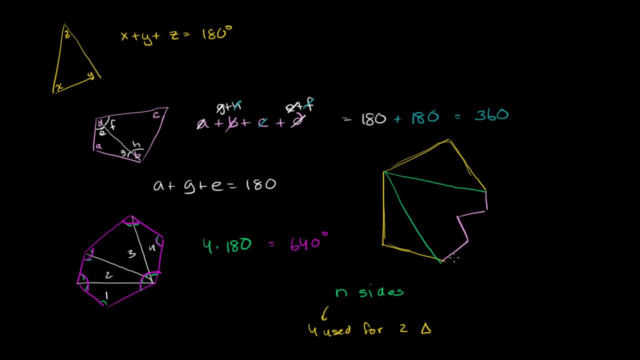 So, for example, if this is so, I have one, two, three, four more sides. So this is a very strangely shaped octagon, But it is an octagon, a very irregular octagon, And so you could have. that's one more triangle. 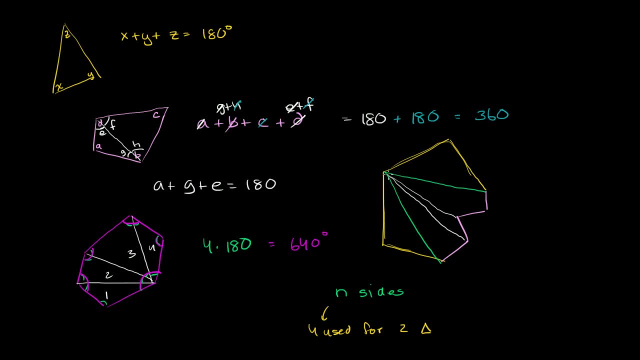 using one more side. Then I have another triangle using another side, And then I have another triangle using that side, And then I have another triangle using this side. Each of the other sides, other than those first four, can help construct another triangle. 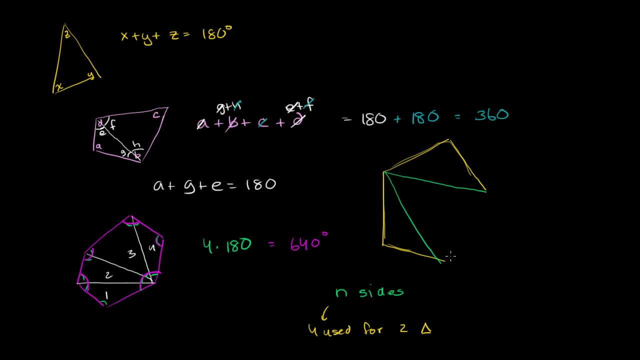 And so the other way to think about it, and you could do this: try to do all sorts of crazy numbers of sides here, And you'll see that once we use these first four sides to create two triangles, every other side we can use to create another triangle. 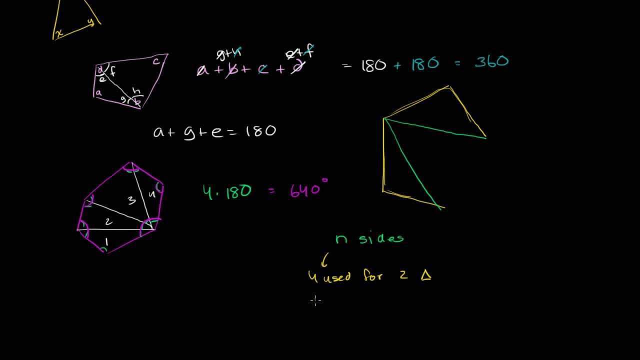 So four used for two triangles, And then every other side can be used to create one more triangle. So if I have n sides, how many triangles can I create? So let's call this: the number. Number of triangles is equal to well, the first two sides. 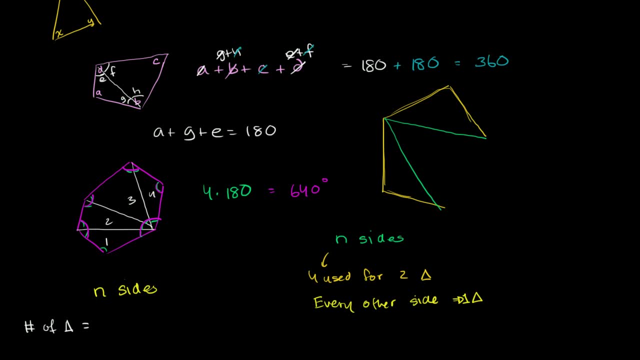 I can make, or sorry, the first four sides. I can make two triangles. So let's say I have at least four sides, So I'm going to have two triangles, So it's going to be equal to two. I'm going to get two triangles out of those first four sides. 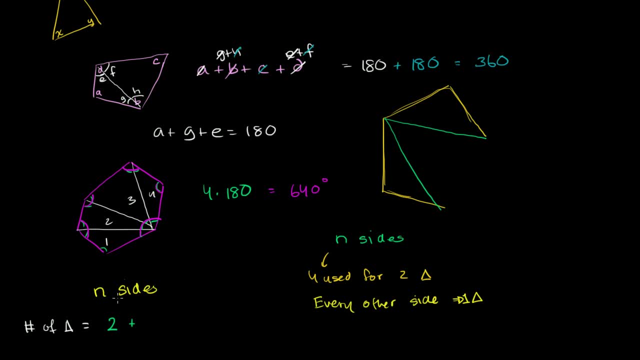 And then however many sides I have after I've used these first four sides, each of them are going to get a triangle. So I've already used, I've already used four sides. I used four of the sides to get two triangles right over here. 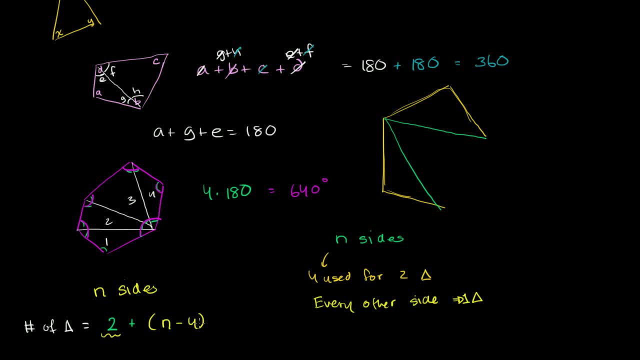 And so then I'm left with n minus four sides, And each of those n minus four sides are going to give me another triangle right over here. So once again, if this right over here, this is a, let's see, this is 1, 2, 3, 4,, 5, 6, 7,, 8,, 9,, 10.. 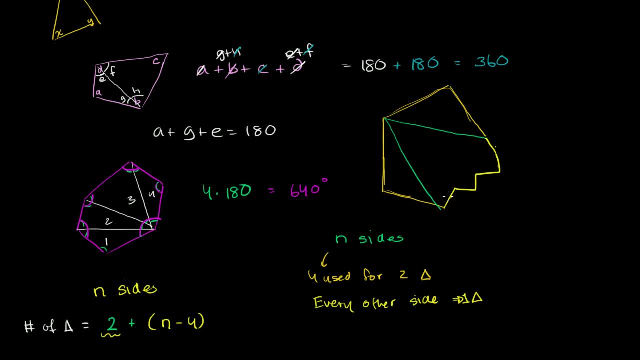 This is a decagon. I use four sides for the first two triangles, And then I have 1,, 2,, 3,, 4,, 5,, 6,, 7,, 8,, 9,, 10.. 4,, 5,, 6 more sides that I haven't used. 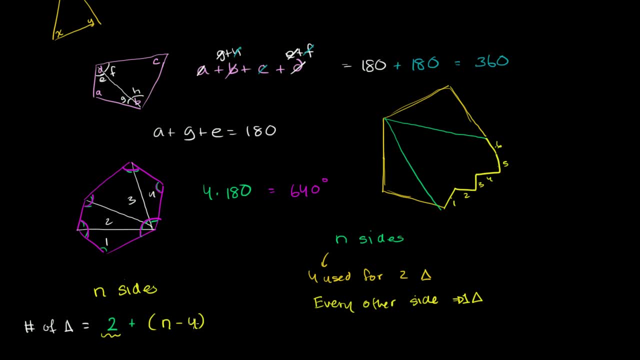 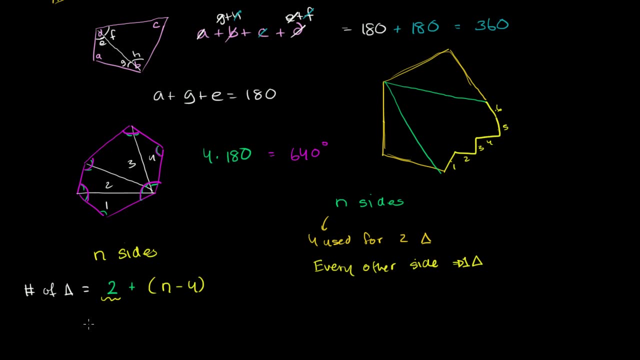 And each of those can form a triangle. So this is 10 minus 4, 10 minus 4 for this decagon. So the number of triangles- if I have n sides, I can just simplify This- is 2 plus n minus 4.. 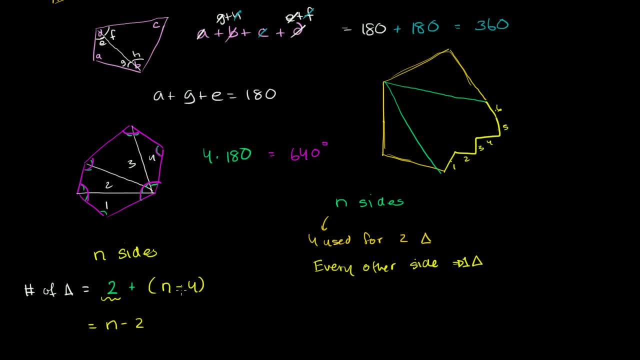 So this is going to be equal to n minus 2.. Negative 4 plus 2 is negative 2.. So the number of triangles is equal to n minus 2.. And we already know from earlier in this video that the number of the sum 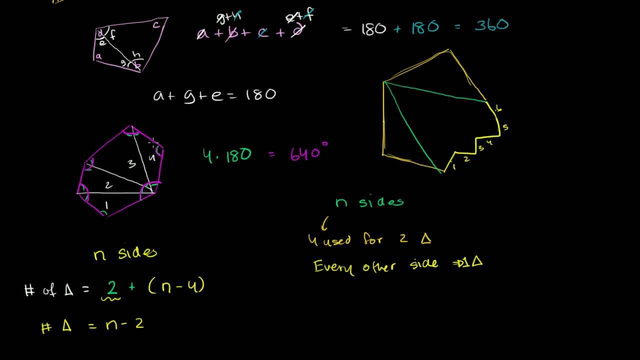 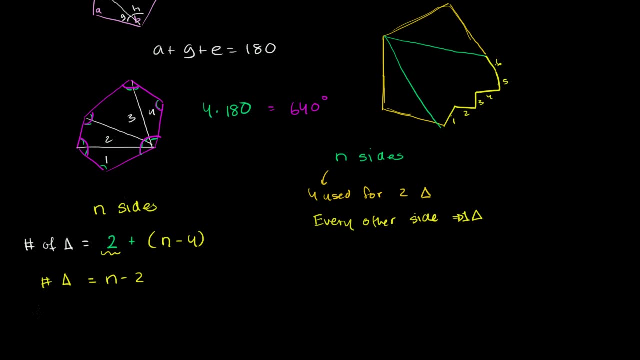 of the interior angles is the number of non-overlapping triangles you can put inside of that polygon times 180.. So we could say the sum of the interior angles are going to be equal to the number of triangles we can create n minus 2, non-overlapping triangles. that 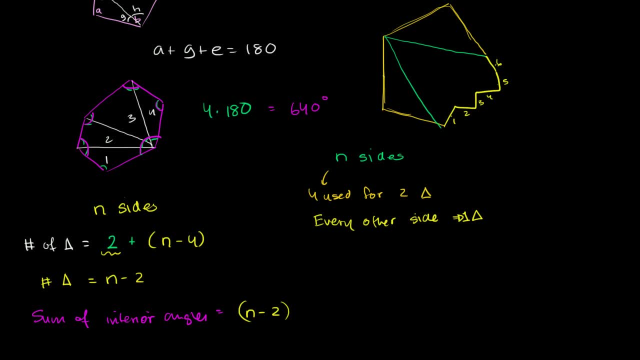 fully cover our polygon n minus 2 times 180 degrees, times the number of degrees, The sum of the degrees per triangle. And so we have a cool little formula here, And I always do forget it and that's why I always re-derive it just by counting the triangles. 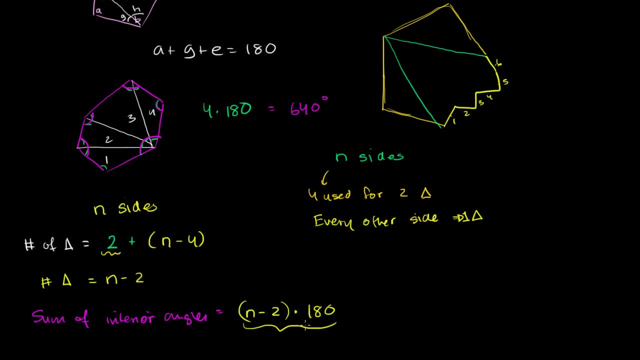 and then multiplying by 180.. But this is cool, because if someone said, hey, I have a 102-sided figure which I won't even attempt to draw, what is the sum of the interior angles of that 102-sided figure?